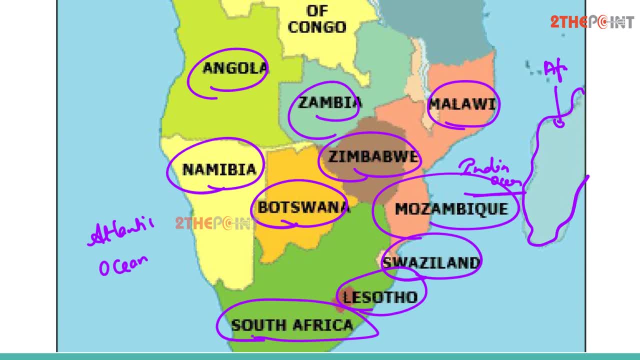 African continent, So it is located to the east of the continent in Indian Ocean. Madagascar. it is said to be the world's fourth largest island and it is similar in area to France. Surrounding Madagascar there are several islands, island states of Seychelles, Comoros and Mauritius. Madagascar once it was. 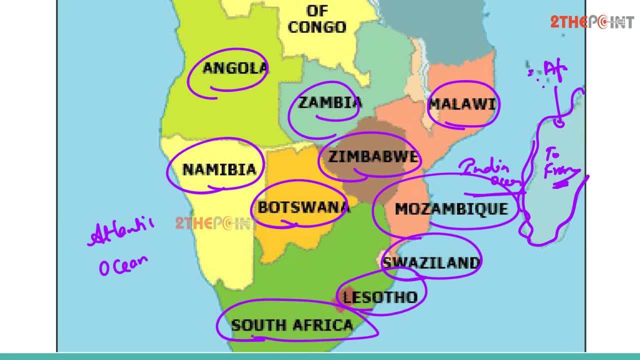 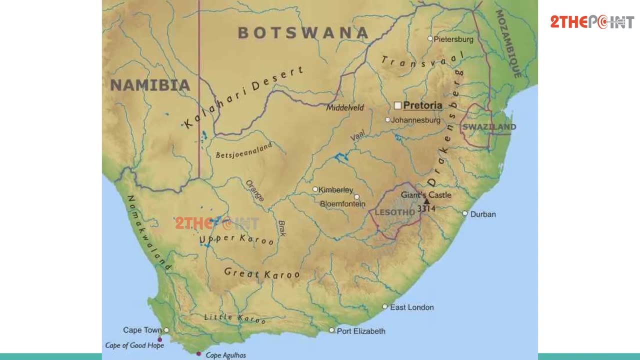 part and part of Africa. but it got separated. it got broke away from the mainland more than 160 million years ago And it developed its own environmental conditions and cultural heritage. Southern Africa: it includes both Sam, unhappy B and Type C climates. The Tropic of Capricorn: it runs straight. 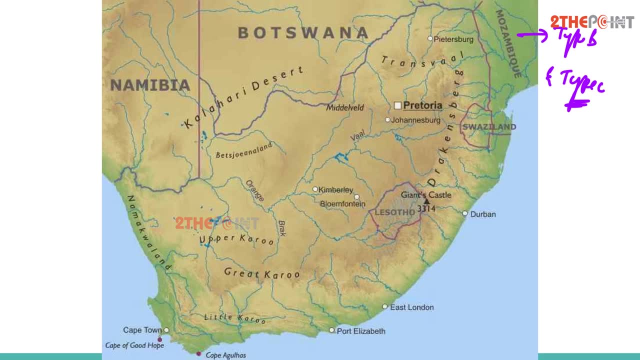 through the middle of the region, indicating the southern position, is outside the tropics and the Calhari Desert, which lies mainly in Bostwana. It is an extensive desert region with an arid mixture of grassy and deep- пож. 200sq. Pastor Anju. with an arid mixture of grassy and deep-Porg- 50sq sq, 60sq, 60sq. In the Calhari Desert it is mainly a bustわna. it is an extensive desert region with an arid mixture of grassy and deep-sp ticked rocks. An Arid mixture of grasses and the formic acid. in the arid desert. The arid mixture of grasses and the arid mixture of arid crystals. An arid mixture of grasses and the arid crystals. It belongs to the local condition of Bostwana. 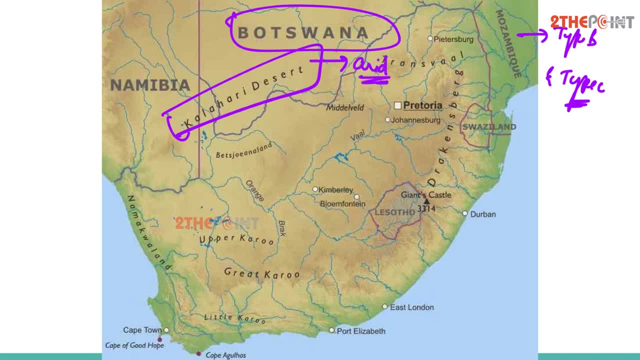 arid mixture of grasslands and sand. so when there is an adequate rainfall, the grasslands- it provides excellent grazing for wildlife. so here the precipitation varies from 3 to 10 inches per year. the Kalahari desert: it is said to be the home to game reservoirs and national parks. the next is Namib desert, and it is 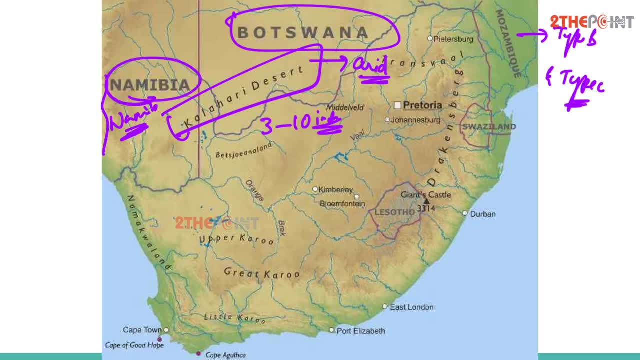 found along the west coast of Namibia, so this receives a very little rainfall and it has moderate type C climate. it is found south of Kalahari desert in South Africa. South Africa is a very large country and it is a very large country and it is a very